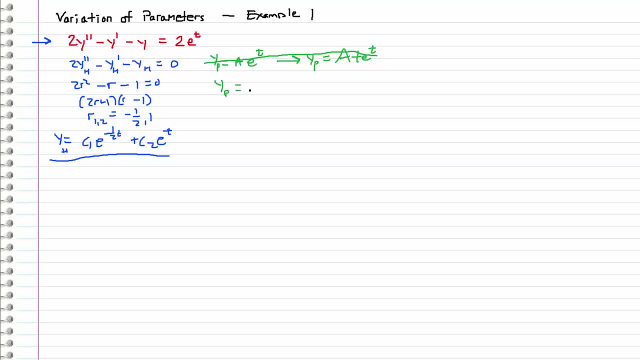 functions. so we would assume a particular solution of the form: u1, which is a function of t times e to the negative one, half t plus u2, which is also a function of t times e to the t, and this should remind you of something, this should remind you of the reduction of order that we used several 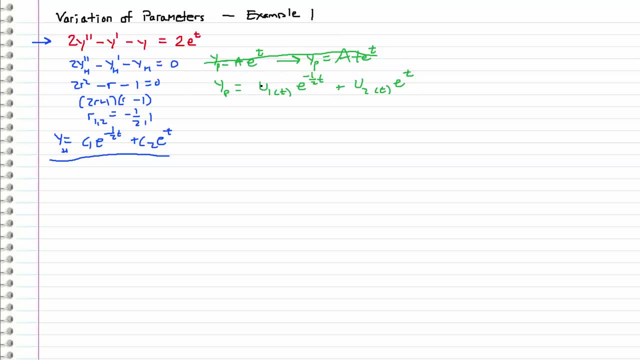 videos ago. but this is like reduction of order on steroids, because we have a u1 and a u2. so the cool thing about variation parameters is that not only do we not have to worry about assuming the right particular solution form, but it also works for a larger class of non-homogeneous equations. 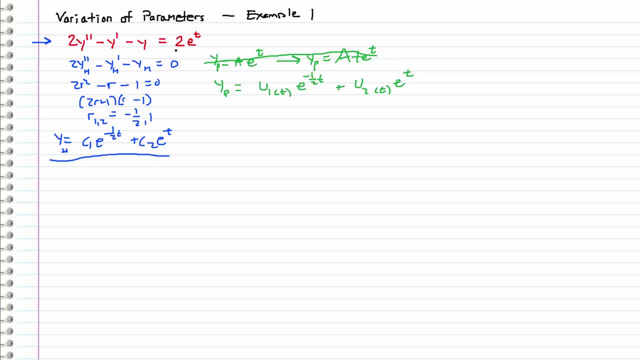 so in the undetermined coefficients we were only able to handle the exponentials, the sine and cosines and the polynomials. but with variation of parameters we can generalize that to be able to handle a lot more non-homogeneous solutions. but anyway, i know we could use undetermined coefficients in this example, but we are going. 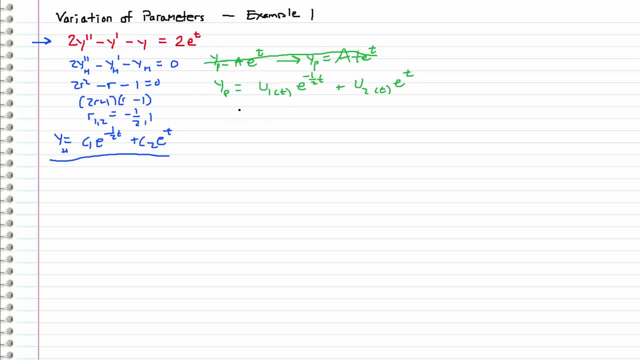 to go ahead and use various parameters instead. so the very next step is to plug in our assumption of yp back into our differential equation and then solve for our unknown functions u1 and u2. so let's go ahead and differentiate yp twice, so we have to use the product rule on here, so we get. 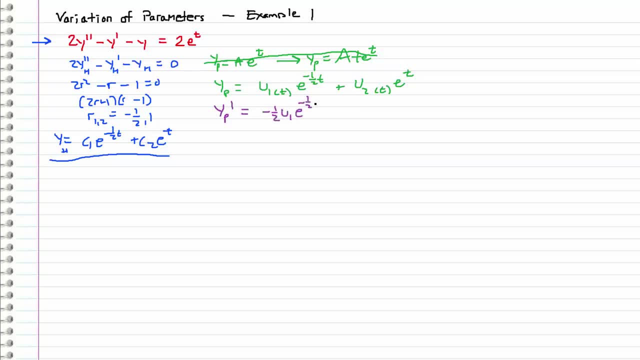 negative one: half u1 e to the negative one, half t plus u1 prime e to the negative one: half t plus u2 prime e to the t plus u2 times e to the t. now there is a very important thing that we need to do next, and that is impose a constraint on our problem. so in yp prime, what we do is we: 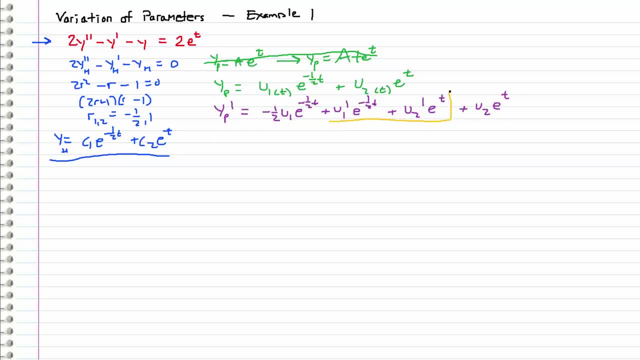 take the two terms that have the primes on them, so the u1 and u2 prime, and we say, okay, let's let these guys sum to zero. and the reason why we do that is to prevent higher order derivatives from the problem, and it's also a necessary constraint that we have to impose so that we can actually 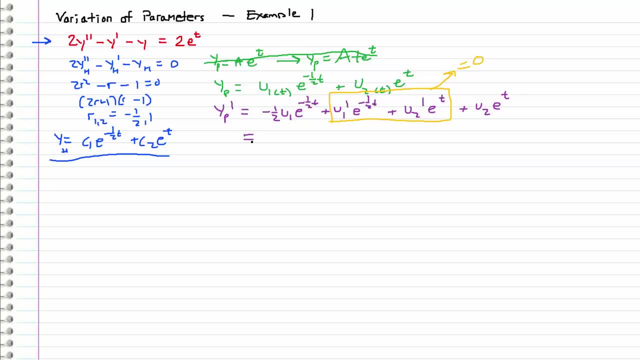 solve for u1 and u2. so, with that said, i am going to go ahead and rewrite yp prime as negative one half u1 e to the negative one, half t, plus u2 times e to the t. these guys they sum to zero. so i'm not. 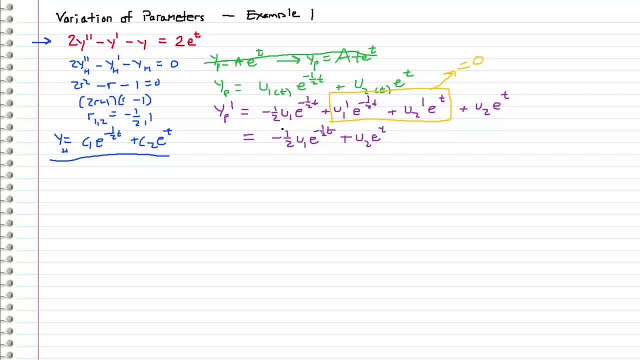 going to worry about them yet. but this fact will come into play later on, so let's keep that in the back of our minds for now. so next, let's go ahead and differentiate again to get yp double prime. so here we get negative one half u1 and u2 prime. so let's go ahead and differentiate again to get yp. 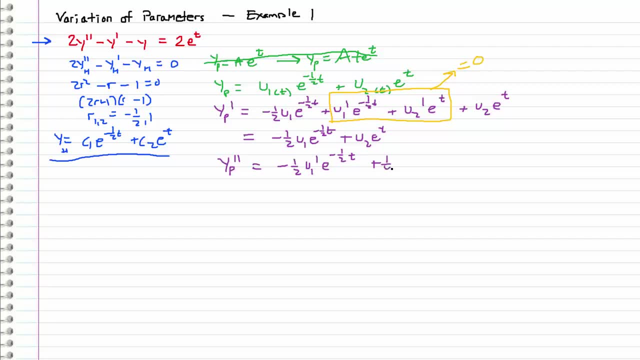 double prime e to the negative, one half t, plus one fourth u1 e to the negative one half t and then plus u2 prime e to the t, plus u2 times e to the t. so we have our three different terms and we can throw it back into our differential equation now. so when we do that we have two times yp double. 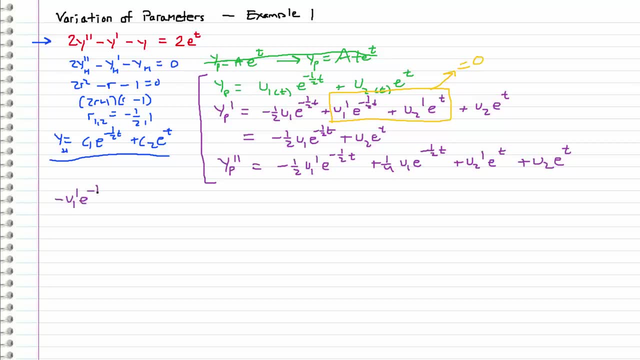 prime. so that gives us negative u1 prime e to the negative one half t plus one half u1 e to the plus two times u two prime e to the t plus two u two e to the t. Then we have a minus y prime. 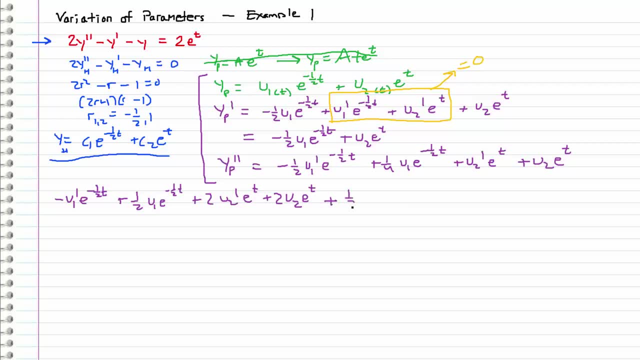 so a minus. actually it becomes a plus one half u, one e to the negative one half t, and then minus u two e to the t, And then we have a minus y, which is minus u one e to the negative one half t. 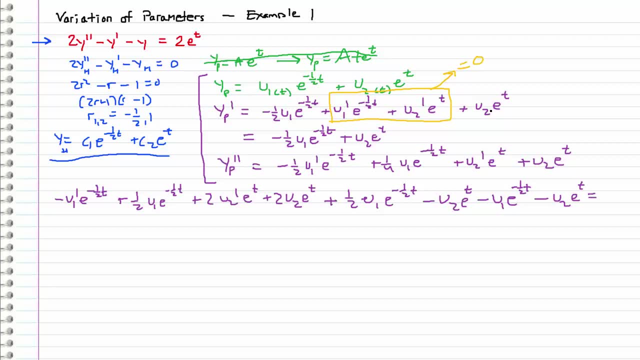 and then minus u, two times e to the t. And all this has to sum up to the right-hand side, the non-homogeneous part, which is two e to the t. So another cool thing about variation of parameters if we have done all of the algebra correctly. 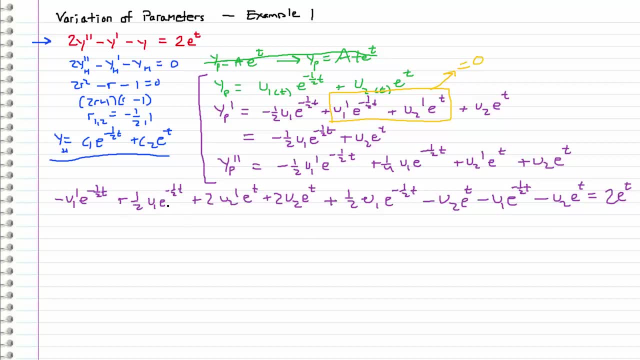 then all of the terms that don't have primes on it should cancel out. So, for example, we have a one half u, one e to the negative, one half t right here. So this guy, and here is another one right here. so now we're at one u, one e to the negative, one half t. 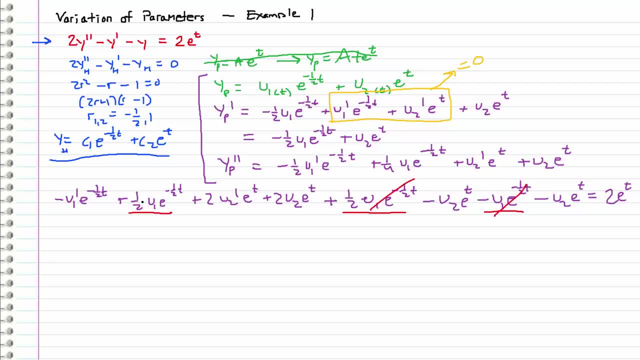 And then we have a minus u one e to the one half t, So all these guys cancel out and we can move on to looking at these guys now. So we have a two u two e to the t, minus a u two e to the t. 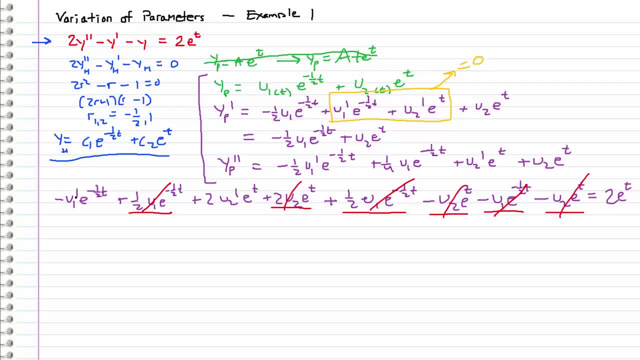 and then minus another one, So all of these guys cancel out as well, And what we are left with is only the terms with the primes, which means that we are on the right track. It's a good way for a mental check to make sure that you're doing this right. 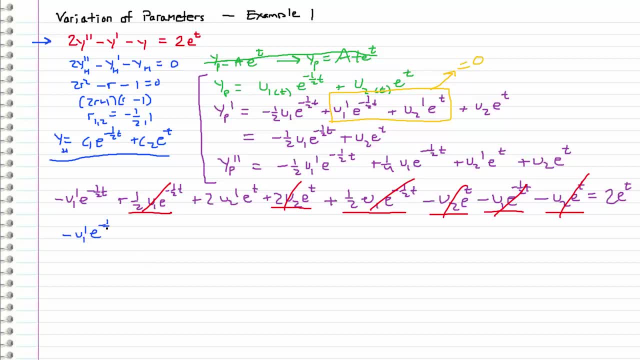 So let's go ahead and rewrite that Negative u one prime e to the negative, one half times t, plus two u two prime e to the t, And this all equals two e to the t. But that's not the only equation that we have. 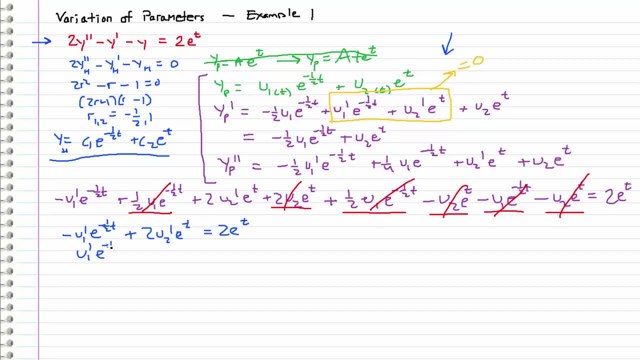 Remember this guy right here We have u one prime e to the negative one half t, plus u two prime e to the t has to equal zero, because that is the constraint that we imposed on this problem. So we have two equations and two unknowns. 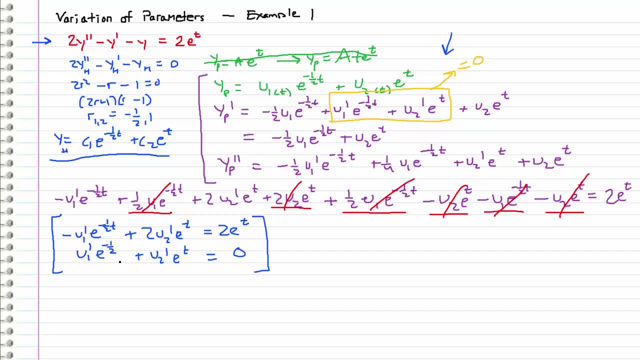 and we can solve that. So the easiest way to go about solving this is by adding the equations together. So if we add them together, what we get is three u, two prime e to the t is equal to two times e to the t. 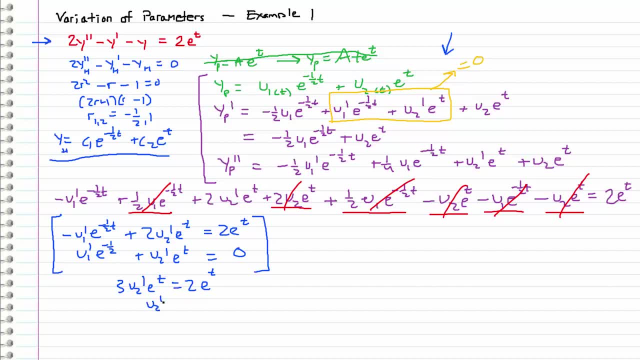 And here we can divide by three e to the t, and what we get is u two prime is equal to two thirds, And then from there we can easily integrate it. So u two is equal to two thirds times t, And I'm not gonna worry about my constants of integration. 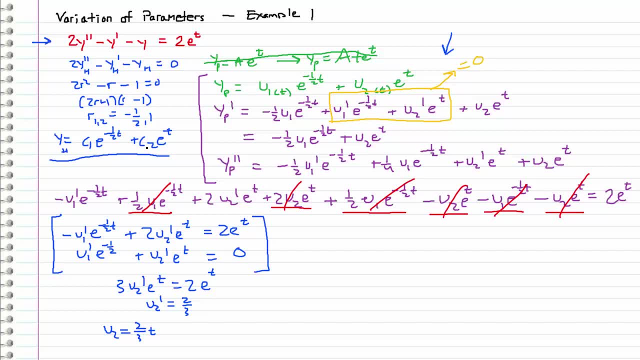 because those are gonna end up getting absorbed up into these constants right here, And I will point that out later, But for now we're not gonna worry about that. So we have an expression for u two and we also have an expression for u two prime. 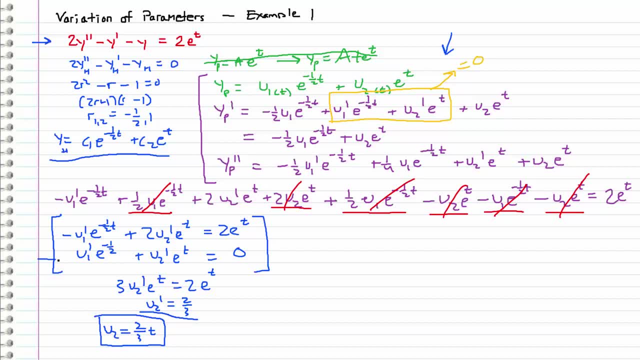 So let's go ahead and use this expression for u two prime and substitute it back in to our second equation. So when we do that, we have u one prime, e to the negative one half t and then plus u two prime, which we determined to be two thirds. 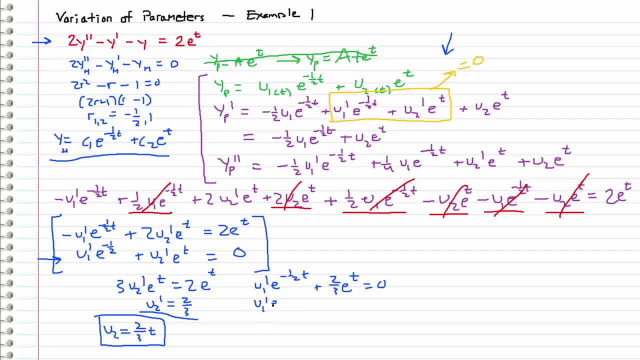 and all this equals zero. So let's go ahead and rewrite this as u one prime e to the negative one half t is equal to negative two thirds e to the t, And then we can divide both sides by e to the negative, one half t. 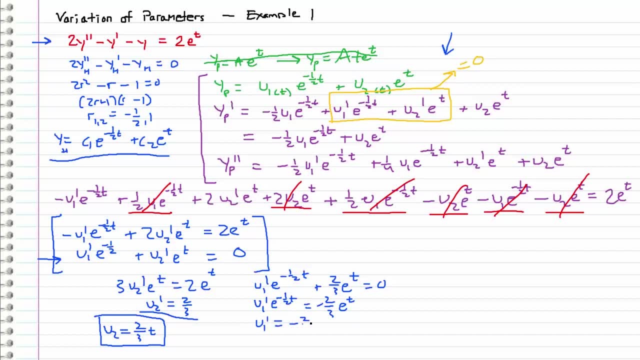 which gives us u one prime is equal to negative two thirds e, to the three halves t, And then from there we can easily integrate it, And again I'm not gonna worry about my constants of integration because again they are going to get absorbed into it. 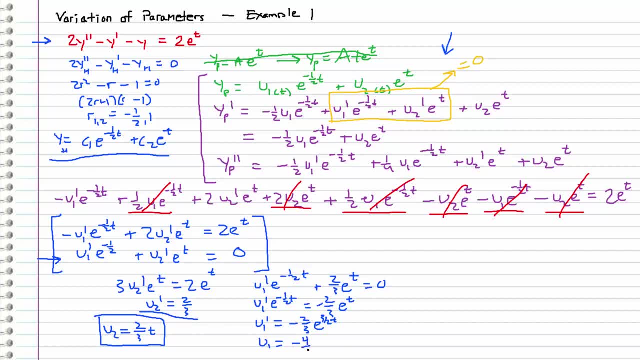 So when we integrate this, we get negative four ninths e to the three halves times t. So we have successfully solved for our u one and our u two, And that means that we are ready to assemble our final solution. So the general solution is always the homogeneous. 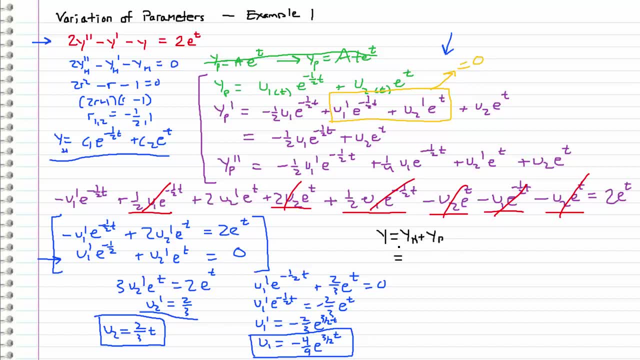 plus the particular solutions, And in this case the homogeneous solution is c one e to the negative, one half times t plus c, two e to the t, And then plus the particular solution which is u one times e to the negative, one half t. 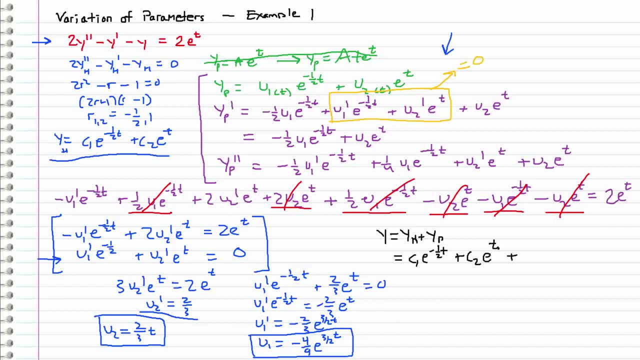 So we have plus our u one which is negative four ninths, so I'm gonna change that to a minus. So minus four ninths e to the three halves t times e to the negative one half t. and then we have plus a u2 times e to the t, and our u2 is just two-thirds t. so plus two-thirds. 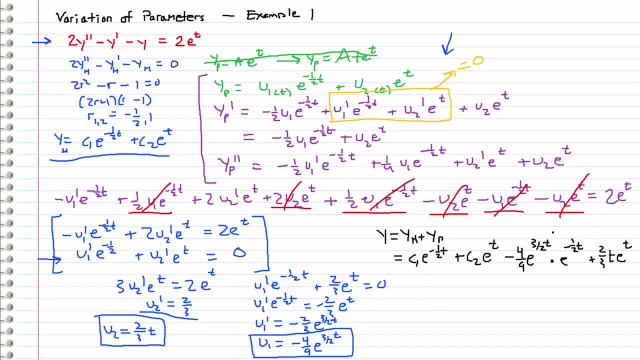 t, e to the t, and we can simplify this third term right here. so i'm going to rewrite this as: c1. e to the negative one-half t plus c2 e to the t minus four-ninths e, and this simplifies to actually e to the t plus two-thirds t, e to the t, and since these two guys are linearly dependent, 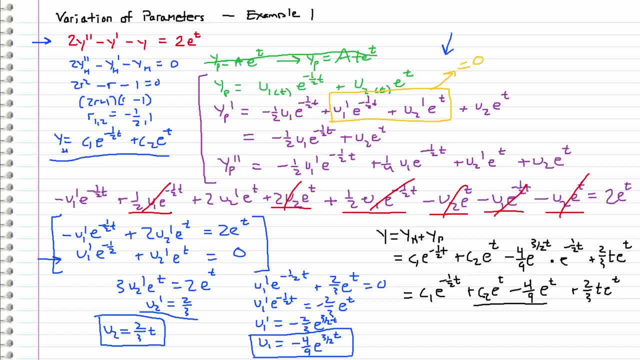 i'm just going to absorb this negative four-ninths into the c2 and i'm just going to go ahead and rewrite our final, final solution as c1 e to the negative one-half t plus c2 times e to the t plus two-thirds times t times e to the t. so this is our final answer and again, just to point out, 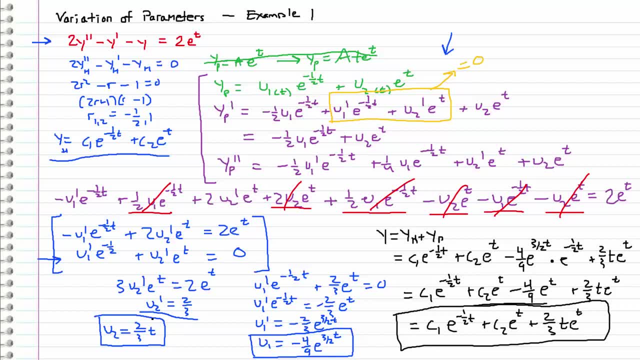 for completeness, if, if i were to keep track of my constants of integration right here, when i integrated u2 prime and integrated u1 prime, if i would have kept up with those constants of integration, then they would have shown up in this equation and would have been absorbed, just like this negative four-ninths. 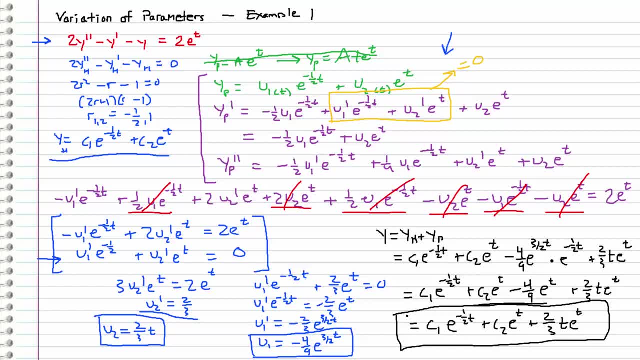 was absorbed into the c2. so there you have it. we have our final answer right here. so also notice that we still end up with this factor of t times this e to the t, just like we would have ended up with it if we modified our particular solution and went with the undetermined coefficients process. 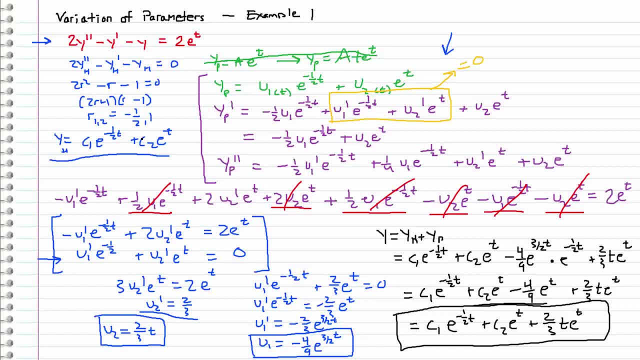 so we didn't have to worry about any of that, since we use various parameters, and we still ended up with the right answer. so, anyway, that's it for this problem and i will see you guys later.